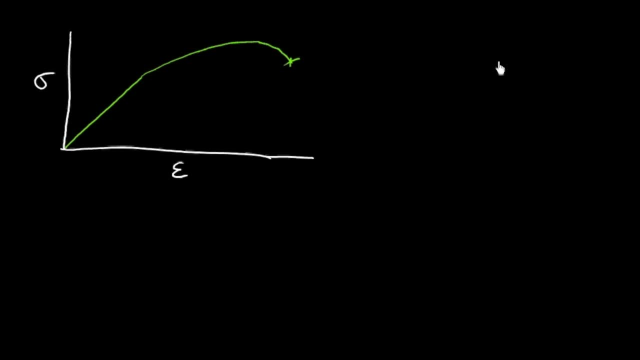 the fracture strength. But what other properties can we determine? Well, first of all, one of them that you may have heard about is the ductility. All right, so ductility has a usage in common language, which is roughly, you know, you might say well. 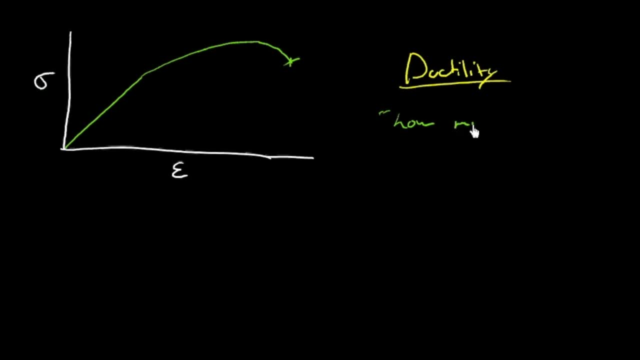 what's ductility all about? If something's very ductile, you might say: well, it describes how much you can stretch something, But of course we know that that's not really accurate enough. Stretch is that referring to elastic or plastic? 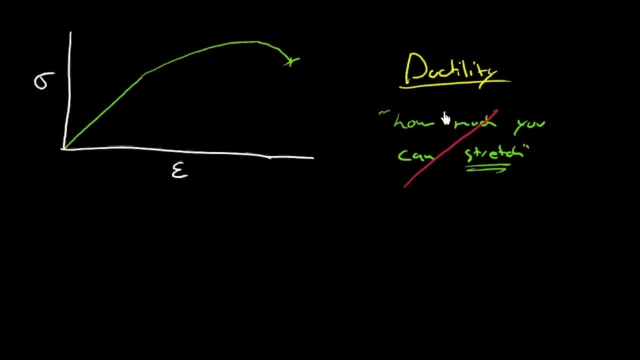 So we've got to be better than that. And in fact I'll tell you Ductility. Ductility is a measure of the plastic strain, So we know clearly it's a strain quantity and it refers to plastic deformation only. 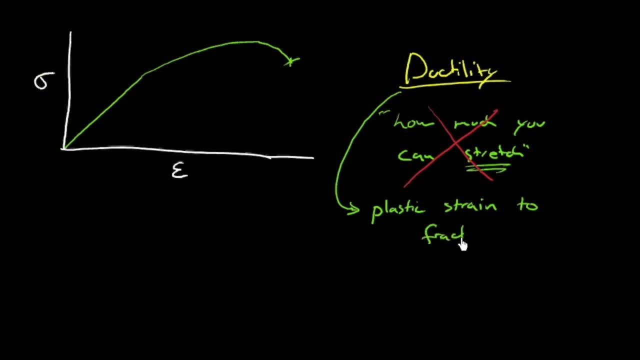 plastic strain to fracture. All right, now we've got something we can work with: Plastic strain to fracture. So let's see. Well, this is the point, This is the point of fracture, That's fracture. So, at fracture, if we unload, we'd 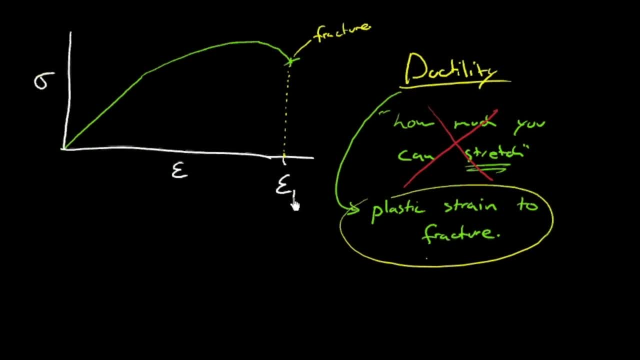 have a value here for total strain. Let me write that in there for you: total strain If we unloaded- so sorry, if we took the total strain there at fracture just a moment before it fractured- that would be our total strain. 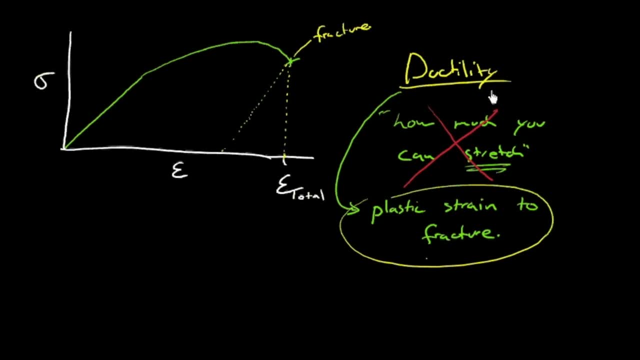 That would be our total strain. That would be our total strain. But what if we unloaded it? Just, you said somehow you knew just infinitesimally before it was going to fracture. Well, we know that the Young's modulus is structure-independent, so it won't change. 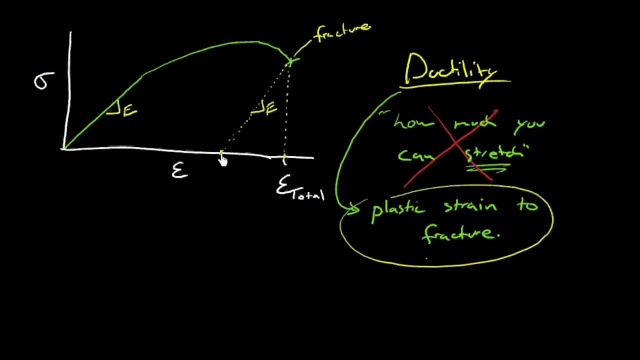 So we would have unloaded that same modulus, which means we'd come back down here to a value on the strain axis, a finite value corresponding to 0 stress. right, It's unloaded, There's no stress on it, but there's still. 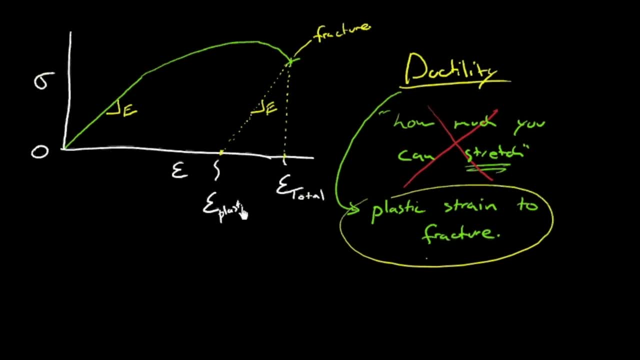 some persistent strain. That means that strain, The strain has to be plastic. That's a plastic strain, which means that this strain in here is elastic. That's elastic, And that makes sense, because what is that? That's the strain underneath this linear unloading portion. 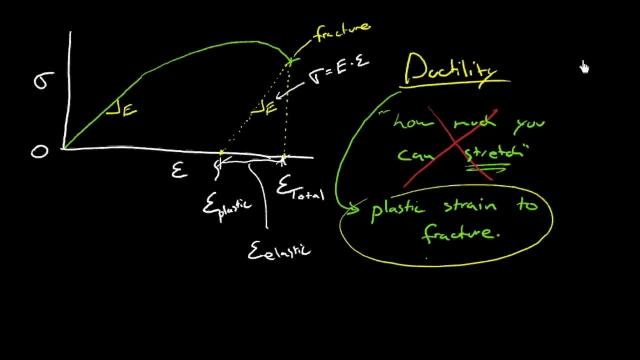 And the unloading portion, if it's linear, is governed by Hooke's law And we know that's elastic because Hooke's law refers to elastic behavior. So if we unload down and we get plastic strain, that plastic strain has got to be the ductility. 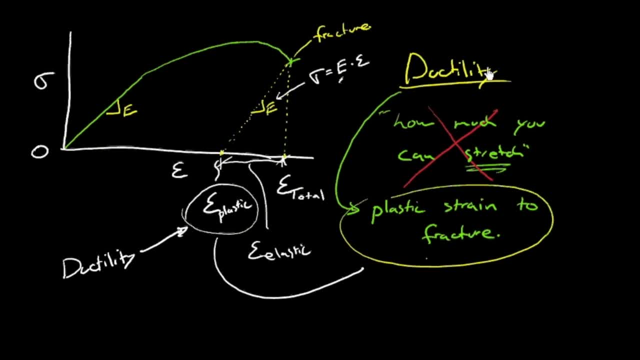 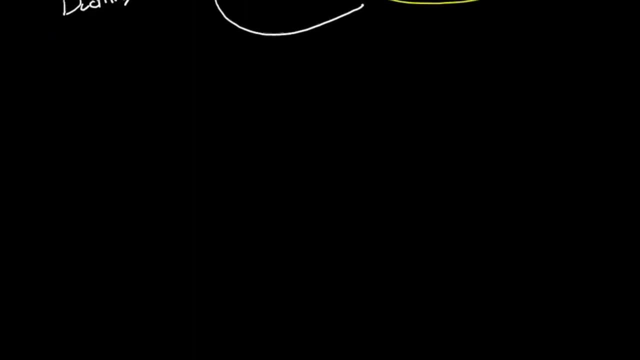 OK, So ductility. you unload that fracture and the remaining strain is the ductility. Another interesting property that we can determine from stress-strain behavior, for a metal or for other material classes as well. OK Is the well, it's called the toughness. 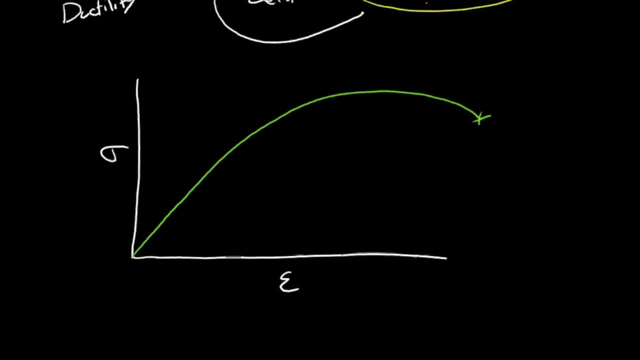 And the toughness is sometimes not such an intuitive quantity. You know you can understand strength, force over area. You get a sense for that. if it's pressure, if you will Even modulus, you can kind of get a bit of an intuitive sense for it. 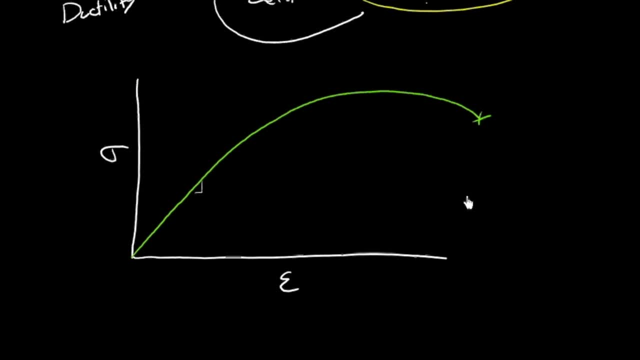 because it's. how hard is it to bend something elastically? It's a little hard, It's a little harder, But the toughness is toughness. I'll tell you what the toughness is: Toughness. Toughness is the energy. 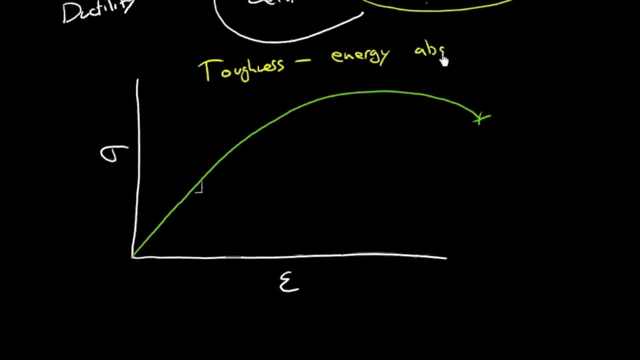 It's an energy term And it's the energy absorbed to fracture, Energy absorbed to fracture. So what we can do actually is integrate, And that is take the area under the curve. So if we take the area under this curve here, 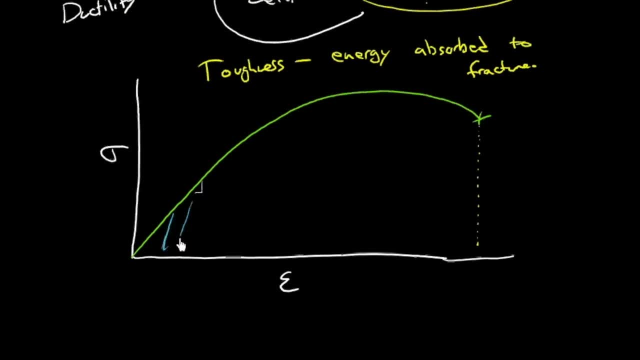 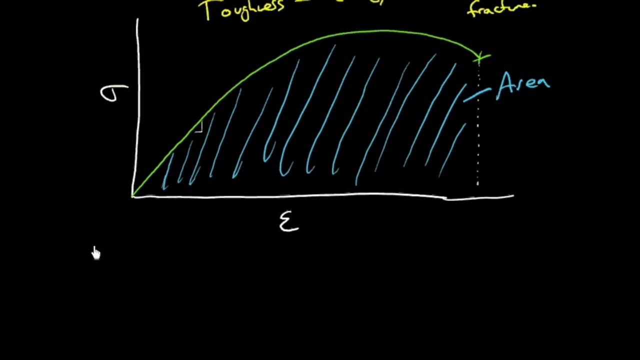 it would be this area here, right, All this area here under the curve is actually the toughness. OK, How do we know that? Well, we could look at it dimensionally. if we're taking the product of stress and strain, Let me look at the dimensions. 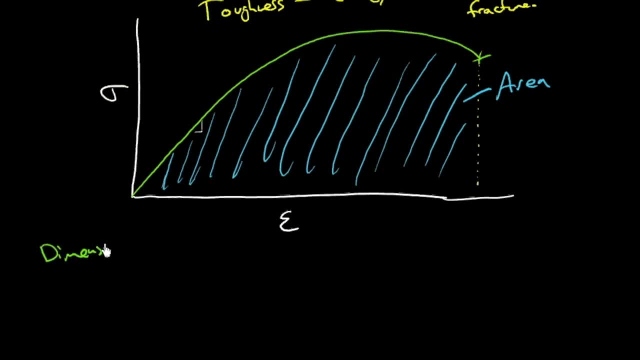 OK, Dimensions Stress has units of pascals, right. And what's a pascal? A pascal is a Newton. Newton per square meter. Well, I can go around living my life multiplying whatever I want by 1, right. 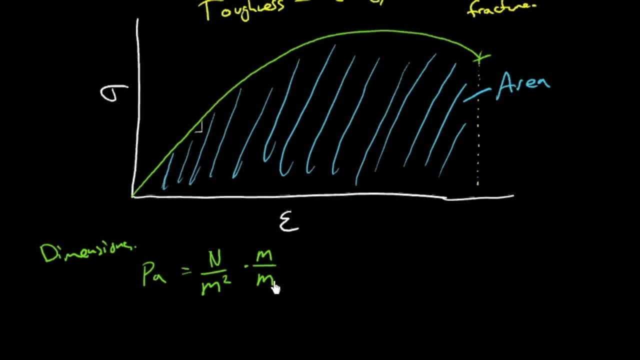 I just multiplied this screen by 1.. You didn't even notice, So here we go. I multiply Newtons per square meter by 1, meter over meter, And I end up with a familiar term in the numerator, Newton meter, And of course in the denominator. 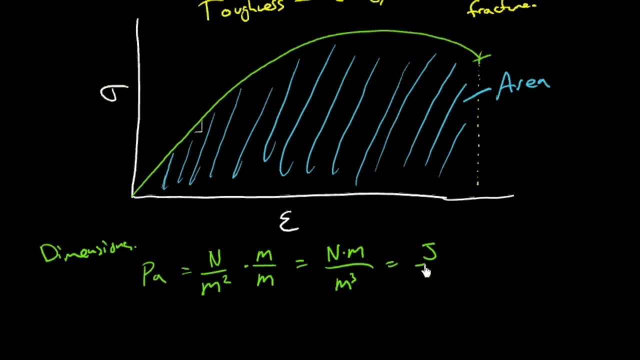 I've got volume units, But what's a Newton meter? A Newton meter is nothing more than a joule, So we've now got joules per volume as units when we integrate under this, And that's great, because we wanted an energy unit. 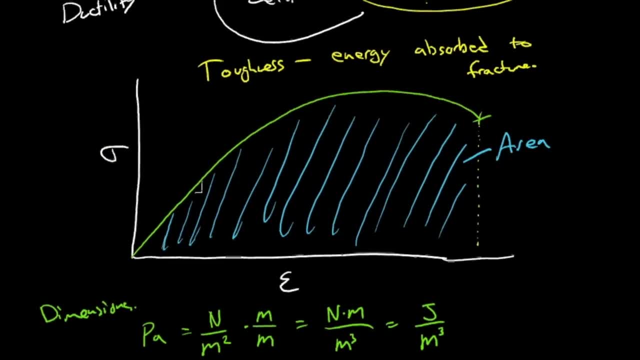 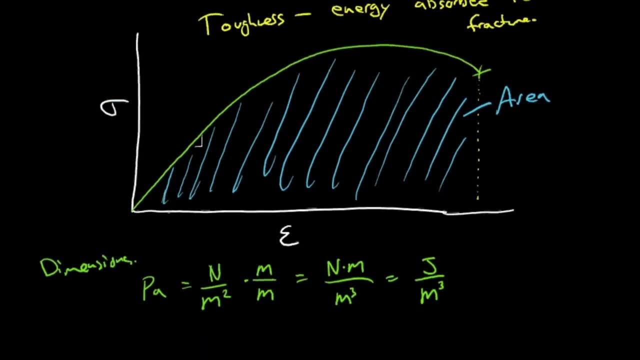 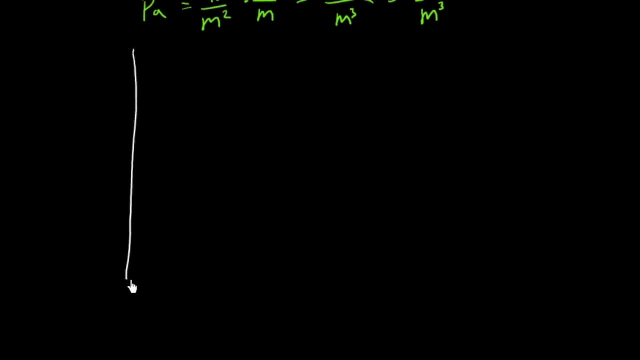 So if we integrate under the entire curve up to fracture, it tells us how much energy went into fracturing that. And that includes- remember that includes- elastic and plastic deformation. Final thing that we can obtain from the stress-strain curve, which is another energy unit, and it's quite useful. 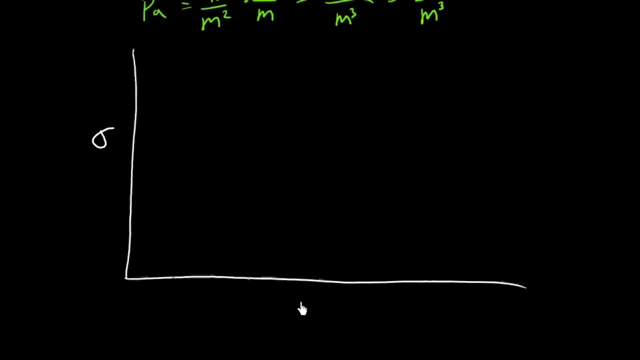 It's a stored energy unit. this time We've got stress and strain, We've got our linear elastic region. plastic deformation and fracture is the resilience, And so the resilience is a measure of the stored elastic strain energy at the yield strength. 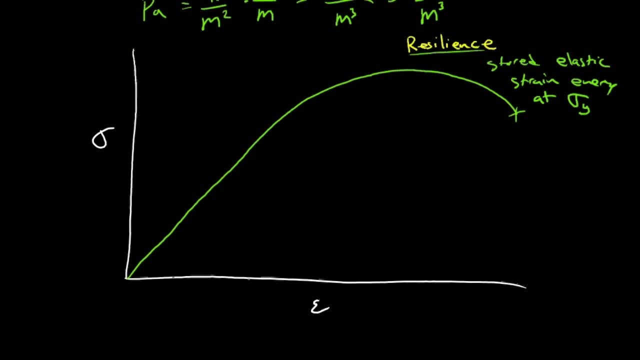 And then we weren't able to do the oru engine in the center. And then we went on to say over- resistance equals velocity. It looks like a bit Dinner đi. And if we down symbol the counter and if we visited 노력ipsing what it says to be 0. 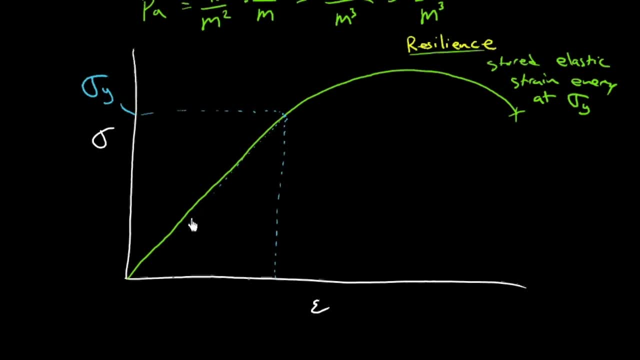 And you can see the difference. It's 1.5, 0.7.. the yield strength: you'd find that you had a little sliver of permanent or plastic strain. Maybe it's close to the 0.2% offset strain. 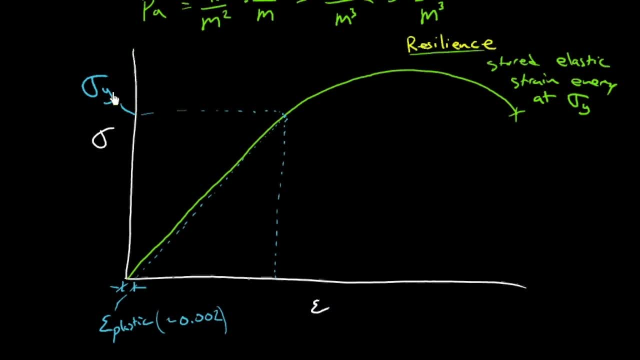 You'd have some plastic strain that had actually accumulated when we had yielding, Even though for practical purposes we say it's elastic before yielding and it's plastic after. you might have a sliver. So we're not going to include that if we're going to be really strict with our definition. 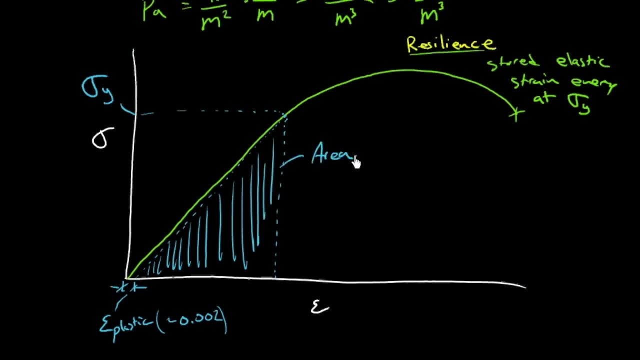 here, And so that area, there is the resilience, And that area actually is just the area of a triangle. It's the area of a triangle And we know that the area of a triangle is 1 half base times height, which in our case, 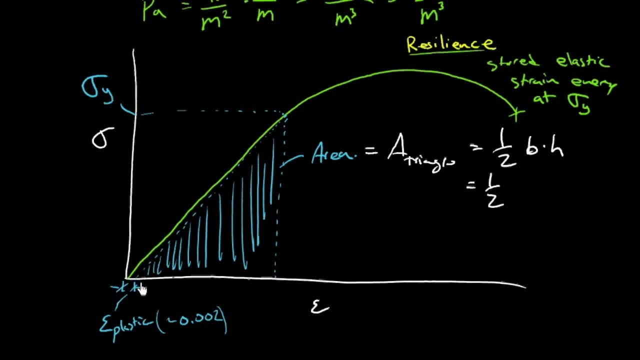 is 1 half of. well, what's the base? The base is the elastic strain, isn't it? And that's good, because we're after the stored elastic strain energy. So we've got strain elastic, And what's the height? 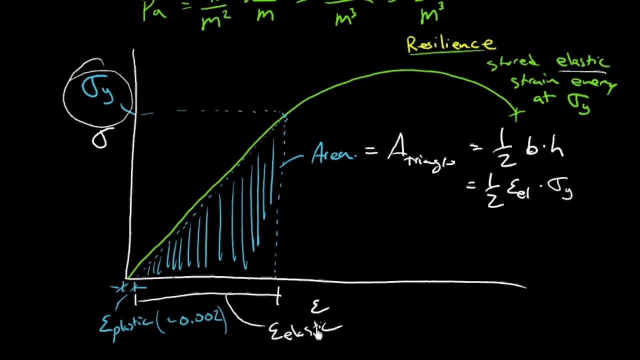 Well, the height is the yield strength, But we can again do better than this, because if it's elastic, it's the strength of the area under this which the strain underneath this linear unloading portion And the linear unloading portion. 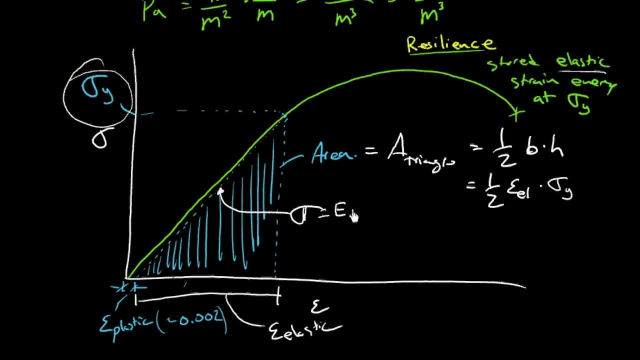 we have a mathematical equation, for We have: stress equals E times strain. It's a straight line. So that means we can say: oh OK, well, that means that the strain is going to be equal to sigma over E. We fire that in here. 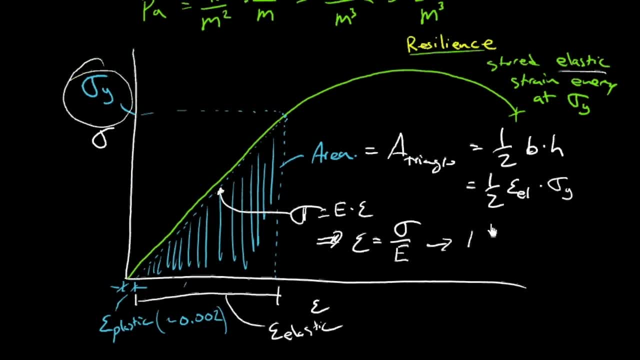 and we find that the resilience is: this is going to be 1 half of sigma And this is sigma yield. That's what we're using here, So that's sigma yield over E times sigma yield And so, at the end of the day, the resilience which we often